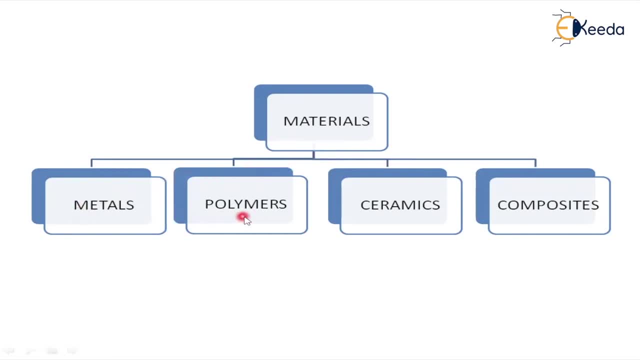 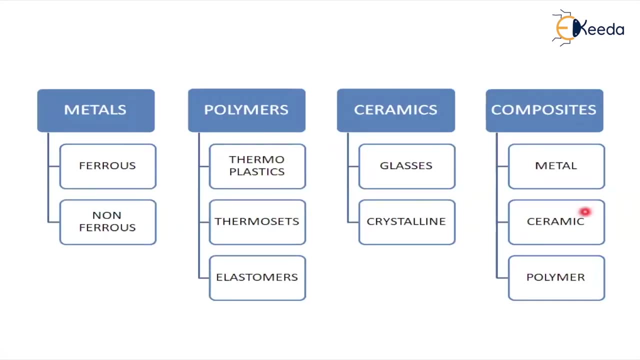 Classified into the following categories: metals, polymers, ceramics and composite. There are sub-classifications for these categories are also available. Follow this diagram to understand the sub-classification of the materials. Now, first one, metals are sub-classified as ferrous and non-ferrous Polymers are sub-classified. 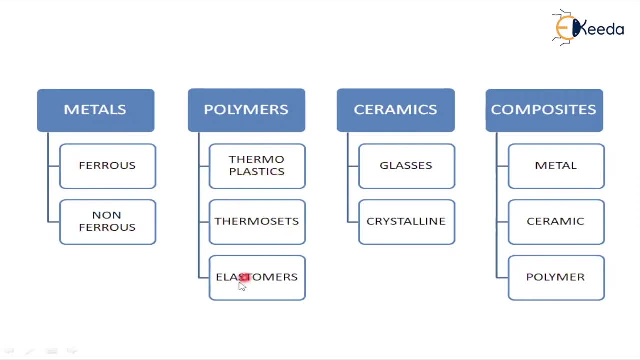 as thermoplastics, thermosets and elastomers. Ceramics are sub-classified as glasses and crystalline Composites are sub-classified as metals. ceramics and polymers means metal matrix composites, ceramic composites and polymer matrix composites. Before going to the details, it is: 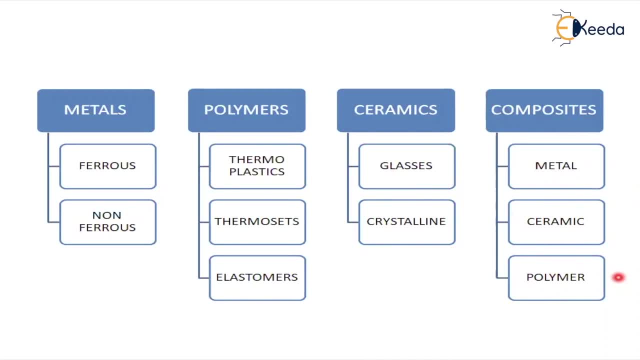 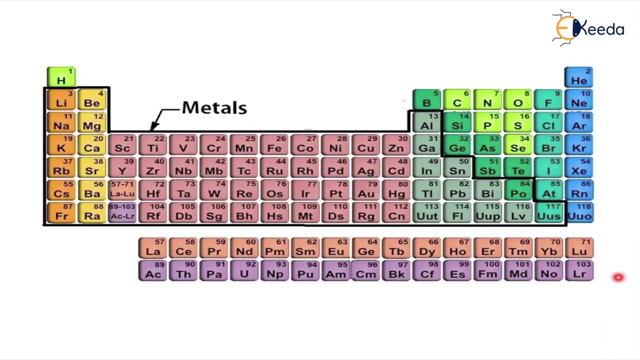 necessary to understand the periodic table. Why the periodic table is necessary. Let me explain. You already know what do you mean by periodic table. The periodic table is tabulation of the chemical elements according to their atomic number and electronic configuration. Just observe the periodic table. If you observe in this periodic table all 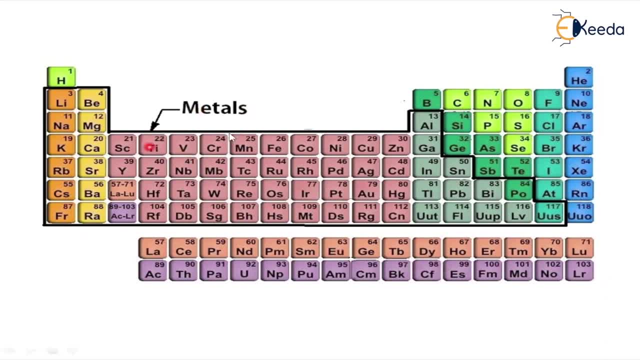 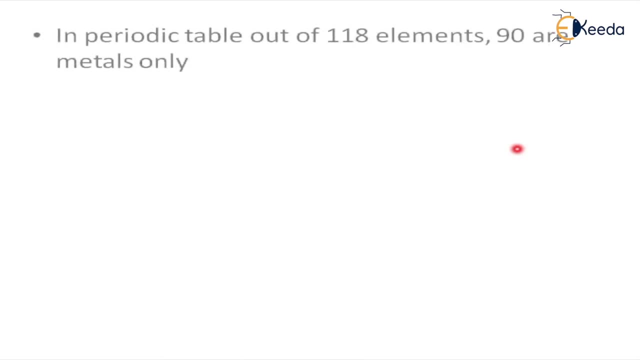 metals are listed on the left side and non-metals means polymers- are listed on the right side of the table Here. just observe the second slide Here in periodic table. if you observe carefully, out of 118 elements 90 are metals only. Just observe carefully one more time. 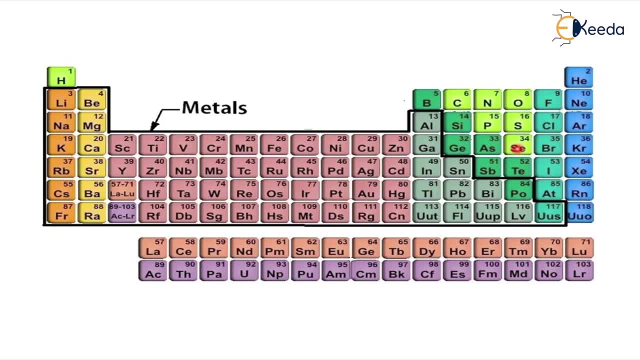 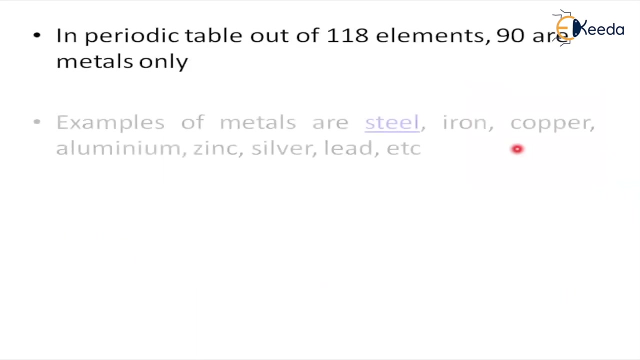 Out of 118 elements, 90 are metals only Here. the examples are steel, iron, copper, aluminium, zinc, silver, lead, etc. So many metals are available which are very famous in our market. Now here these metals are further divided into ferrous and non-ferrous. 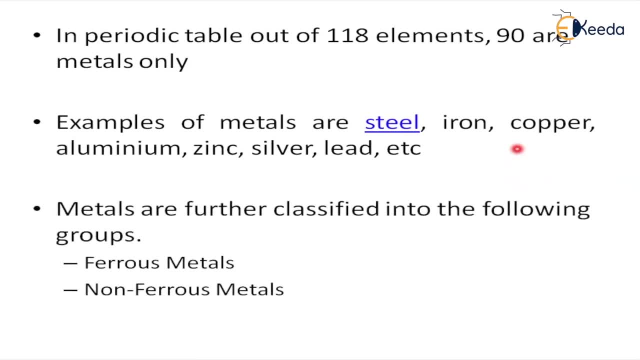 So you can think of such metals as ferrous and non-ferrous, as removed Here. these metals are further divided into ferrous and non-ferrous. now let us discuss. what do you mean by ferrous metal and non-ferrous metals? What is the 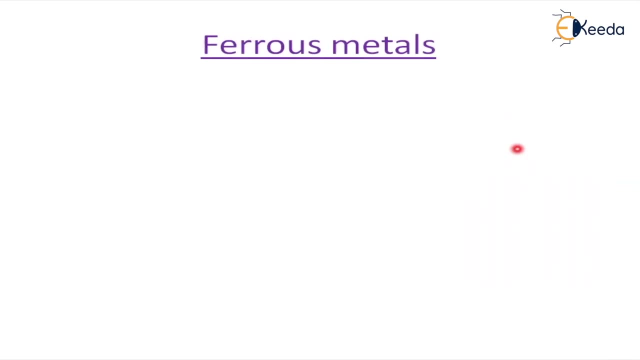 mean by ferrous metal. What are the salient features of ferrous metal? Let me discuss like this. The first point is: ferrous metals are rich in iron means the iron composition is very, very important and it is having maximum percentage in ferrous metals. Steel is the. 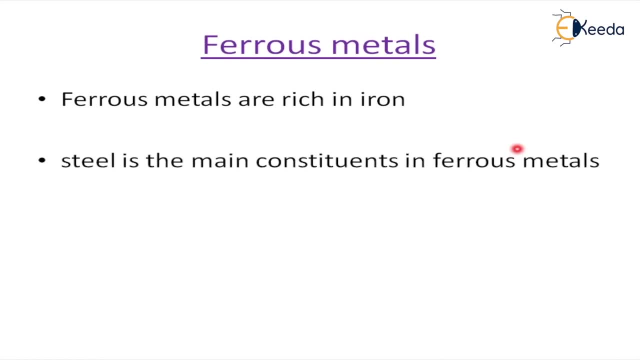 main constituents in ferrous metal. Various examples, if you observe, for the ferrous metals are cast iron, carbon steels, alloy steels, stainless steels, tool steels and die steels. The second classification- that means next classification- is ferrous metals. The second classification- that means next classification, is ferrous metals. 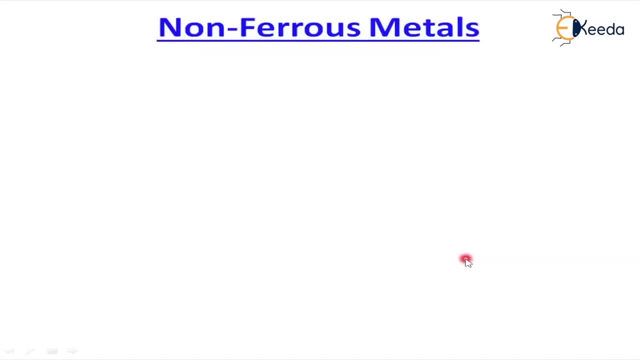 The third classification- that means next classification- is ferrous metals. These metals actually don't have the iron as the main composition. that is the main point to understand non-ferrous metals. For example, if you take the example of aluminum, copper, These metals are not. 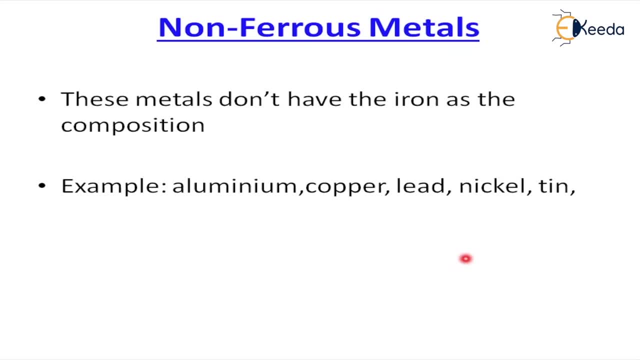 having ferrous Lead, nickel, tin, titanium and zinc. So these non-ferrous metals are very, very famous in the market and very much useful. If you observe aluminum, aluminum is the most non-ferrous metal which is abundantly available in the earth crust. 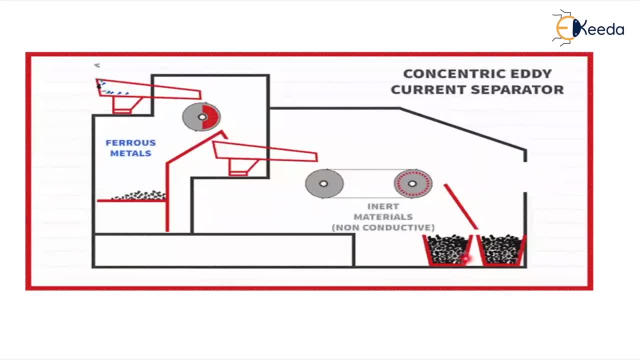 Now observe what is happening in the industry. In any industry in general, ferrous and non-ferrous metals are separated like this And, if you observe, inert materials are also collected here. And here is a technique that is concentric eddy current separator. 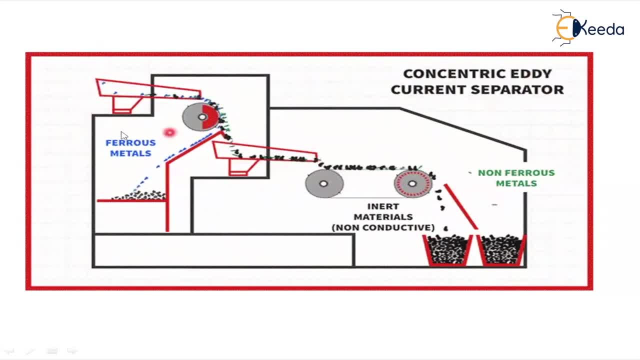 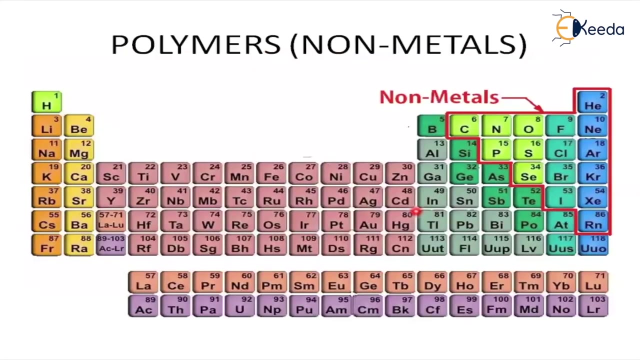 This is the technique they are using. Just observe this picture carefully. Ferrous metals are collected here, Non-ferrous metals are collected here, And inert metals are collected here. Now let us discuss the polymers. What do you mean by polymers? 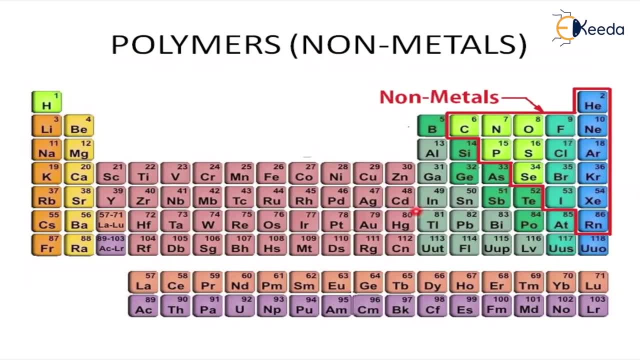 Why polymers are very much important in the market. Now this is the second classification of materials, That is, non-metals polymers. That means the other name of the polymers is non-metals. If you observe carefully, non-metals are occupied. 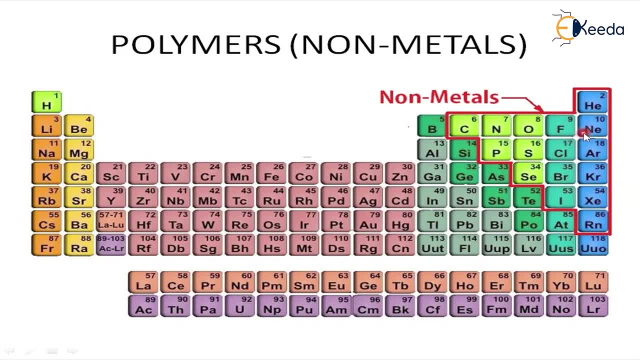 The right side portion of the periodic table. Here, what do you mean by polymer or non-metal? Non-metal is referred to the chemical elements which are volatile, insulated to heat and electricity, and lack of the metallic attributes. Most of the non-metals are gases only. 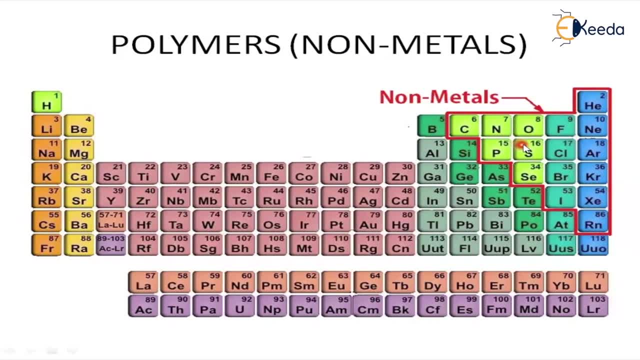 In the periodic table. they are represented under polyatomic, non-metal, diatomic non-metal noble gases: carbon, phosphorus and sulphur, like this. So many non-metals are observed here, See the periodic table. And so here, if you observe carefully, only non-metals are very few. 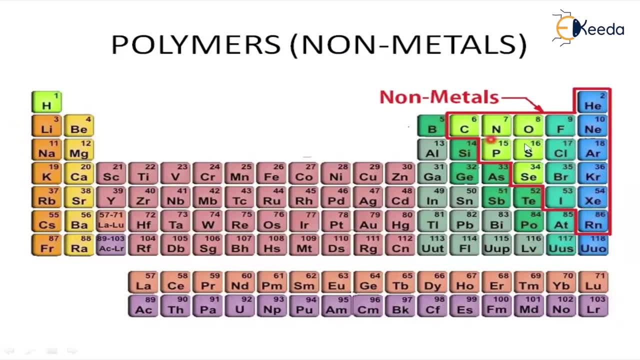 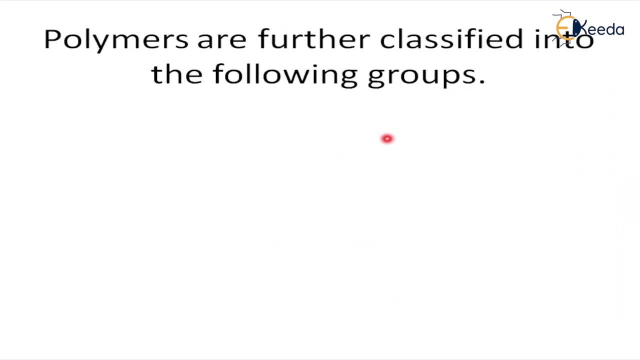 Just observe the periodic table. All these are non-metals only: Polymers. mer means one unit, Polymer means many number of units get together. Now this is classified. Polymers are classified into the following groups, That is, thermoplastics, thermosets, elastomers. 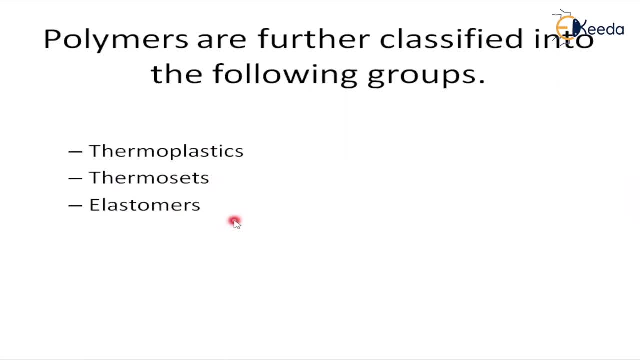 In this video I am just discussing classification, So that's why I am not giving a detailed explanation of all these. In the next coming video I will explain the total properties. In this video I am just concentrating on classification Now. the polymers are classified as thermoplastics, thermosets and elastomers. 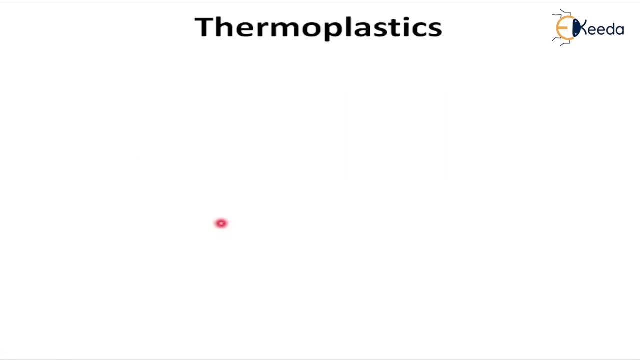 Now let us discuss thermoplastics. So what is thermoplastic And what is the difference between thermoplastic and thermoset? A polymer that can become moldable to a specific heat, then that gets solidified upon cooling, are known as thermoplastics. 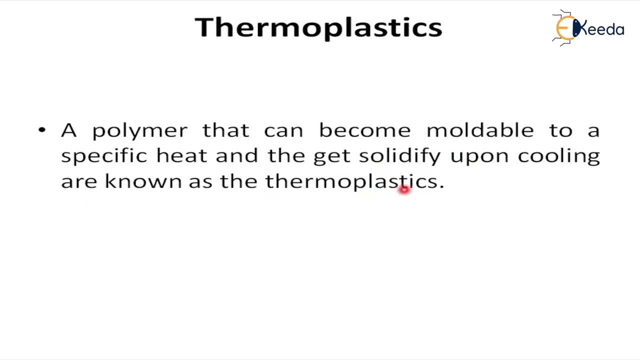 And the second salient feature is very, very important. So these thermoplastics can be remolded or reshaped many times as we want. This is the main feature for any thermoplastic, So they are recyclable polymers. 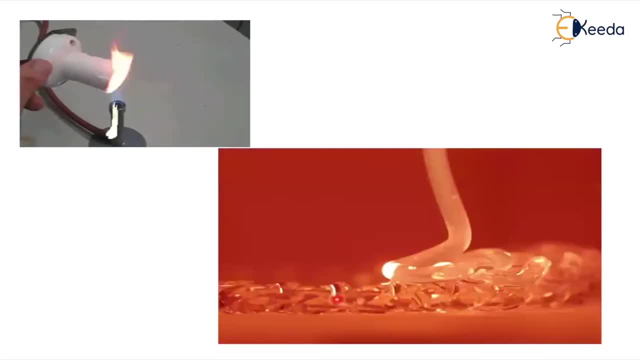 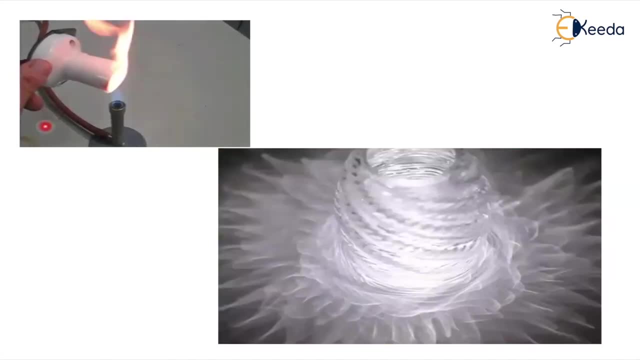 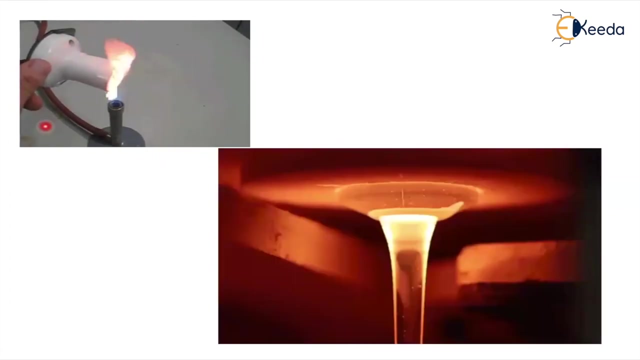 Please observe the two figures. These two figures here, these two figures, shows how thermoplastic material behaves. So that means even that is by giving specific heat and they will get solidified upon cooling And again we can utilize, we can reshape, remold it. 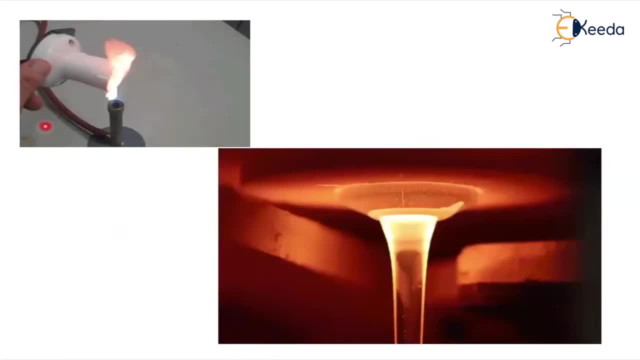 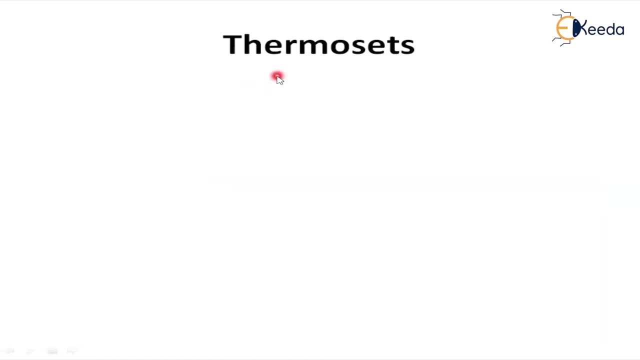 That is the main property of the thermoplastic. Now the second type is thermosets. So what is thermoset And what is the difference between thermoplastic and thermoset? So here, these thermosets are polymers only. 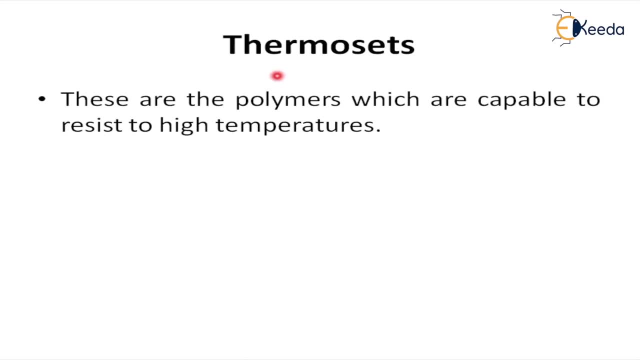 but which are capable to resist to high temperature. That is the main advantage of thermoset. This is the main difference between thermoplastic and thermoset, And the second main advantage of thermoset is once thermosets get hardened. 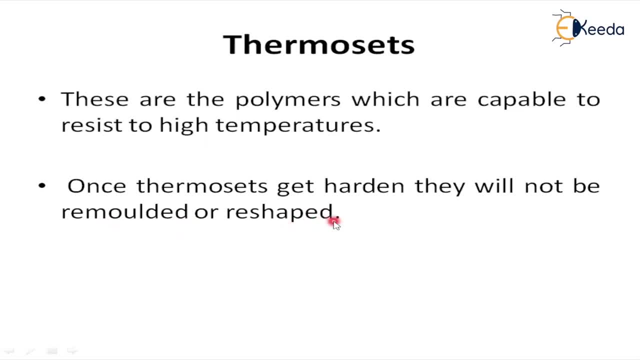 they will not be remolded or reshaped, Even though it looks like a disadvantage, but it is the advantage for some materials. So these are not capable to recycle. This is the main feature of thermoset: capable of resistance to the high temperature. 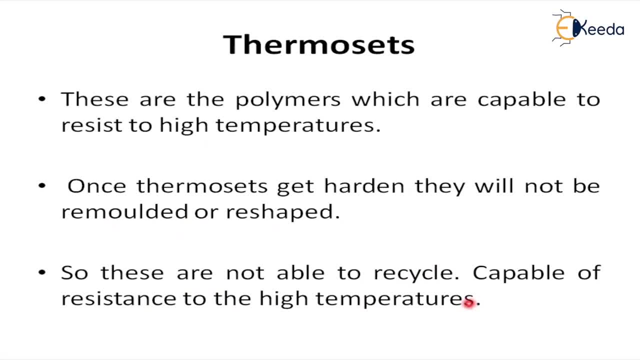 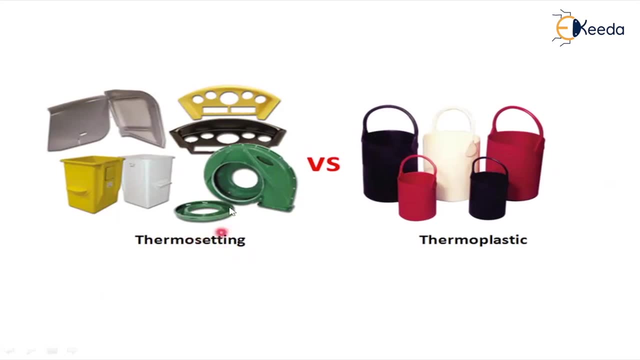 This is another feature of the thermoset. So that means once it is formed we cannot be able to recycle. So this is the main feature of the thermosets. You can observe the various products of thermoset and thermoplastic. 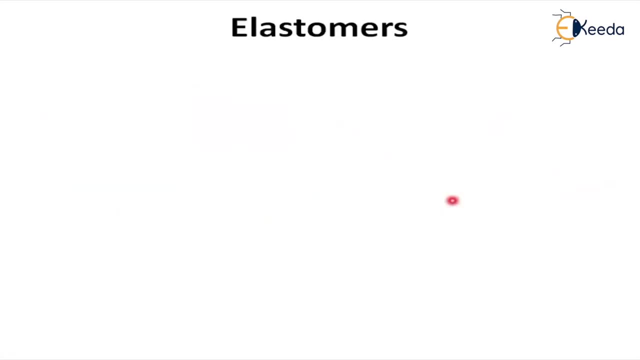 The next type in polymers is elastomers. What do you mean by elastomers? Is it a different polymer? Yes, it is a different polymer compared to thermoset and thermoplastic. The elastomer. what do you mean by elastomer here? 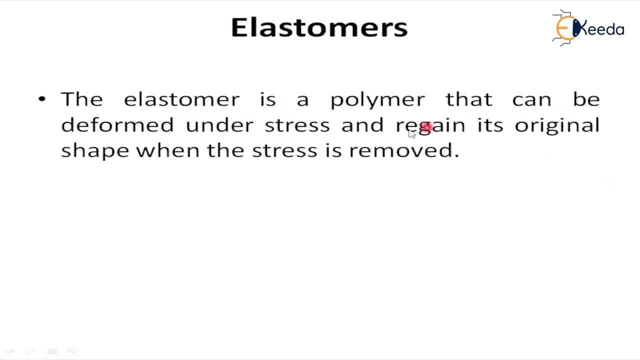 Please observe the definition. The elastomer is a polymer that can be deformed under stress and regain its original shape when the stress is removed. Means, if you remove the stress, automatically it will regain its original shape. Simply we can say that. 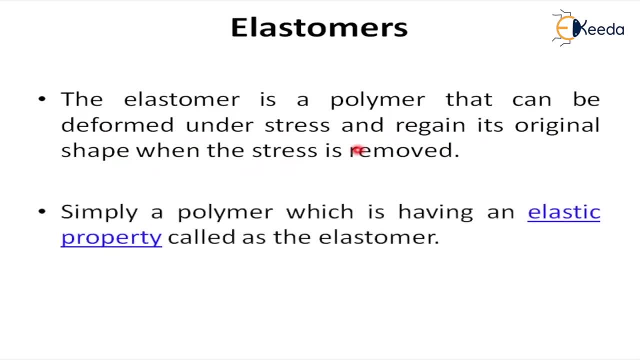 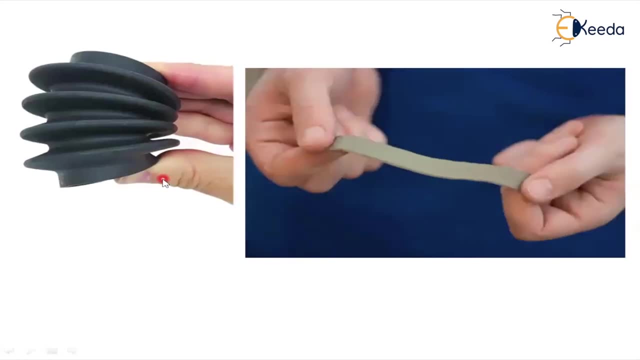 polymer which is having an elastic property is called as the elastomer. This is a simple definition for the elastomers. Now see the figures here. These two figures show how the elastomer works. After removing of the load, again it is getting into the original shape. 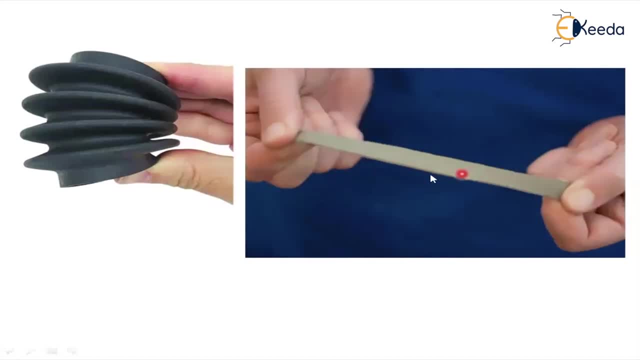 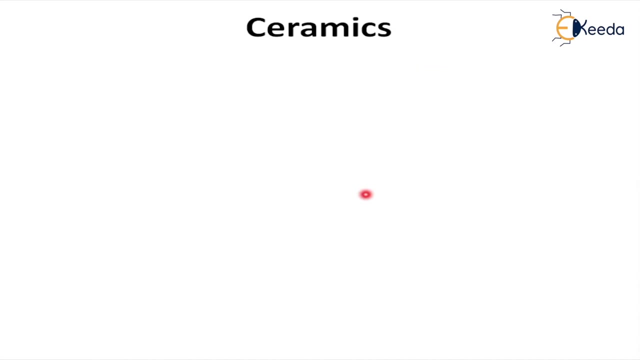 That is the main feature of the elastomer. The next classification, the third classification of materials is ceramics. So what is ceramics? What is the importance of the ceramics in the market Here? it is a must to know about ceramics. Why? Because 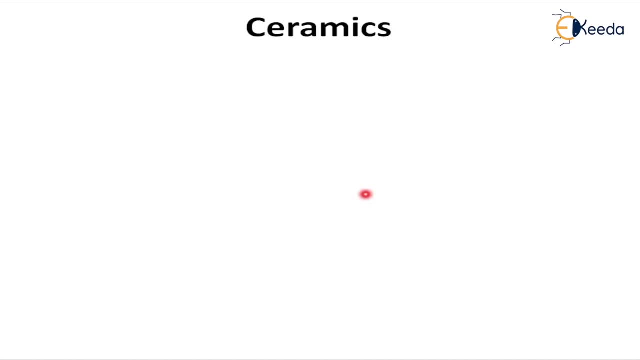 most of the houses or any advanced materials nowadays, they are utilizing ceramics only. Without ceramics, you cannot think about houses now, So that's why ceramic is a very, very important material in the market. Now let us discuss some salient features about ceramics. 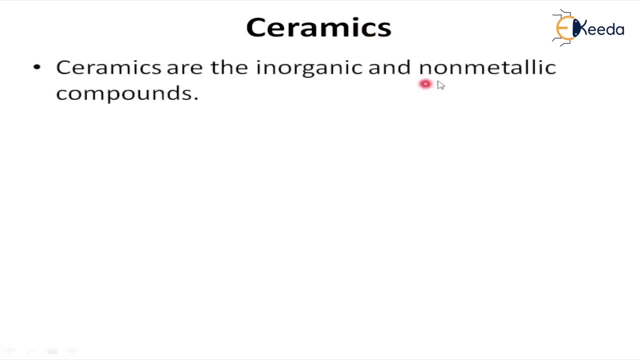 Ceramics are the inorganic and non-metallic compounds. Examples, suppose: if you take the examples, most of the examples are plates, tiles and toilets. Most of the toilets are built with ceramics, only Ceramic tiles, And these are further classified. 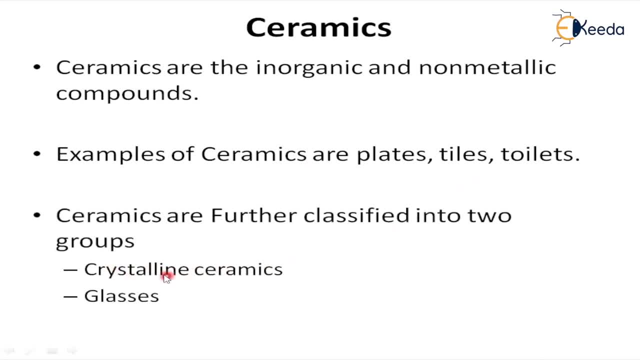 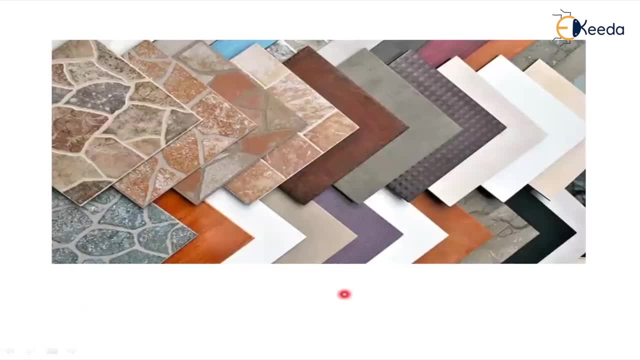 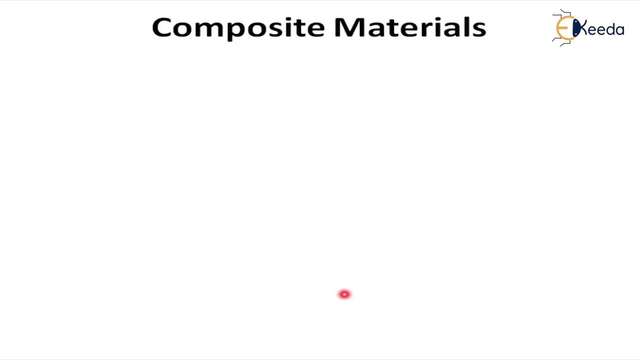 if you observe the classification, these are further classified as crystalline ceramics and glasses. The best example of the ceramics is tiles. only You already know what is the importance of the tile in our regular life. Now the next important material is composite material. 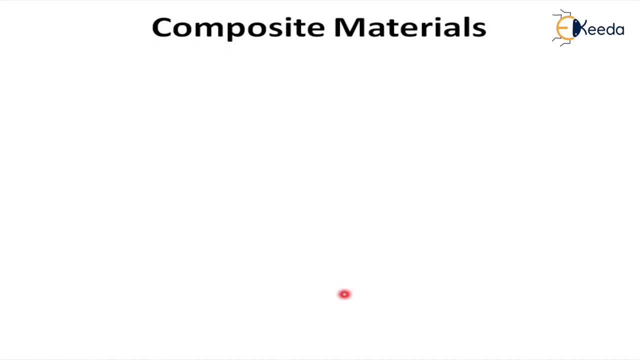 This is the last classification of the material. The most thrust area for research and most useful materials compared to any other material in the market is composite material only. Let us discuss a few words about composite material. What do you mean by composite material If you observe the definition? 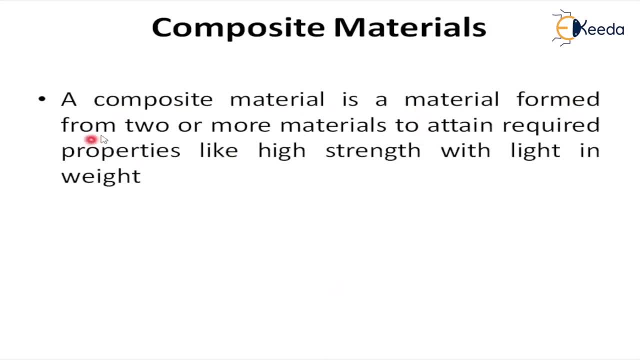 a composite material is a material formed from two or more materials- This sentence is important- Two or more materials to attain required properties like high strength with light in weight. So exactly what do you mean by composite material? So that means you can form with two or more materials. 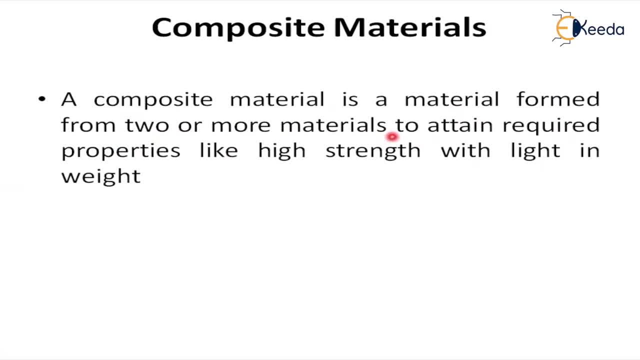 But the important, the main intention of the composite material is to produce high strength with light in weight. That is the main intention. Example: if you take the example, the best example is plywood. only You are seeing the plywood in our regular life. 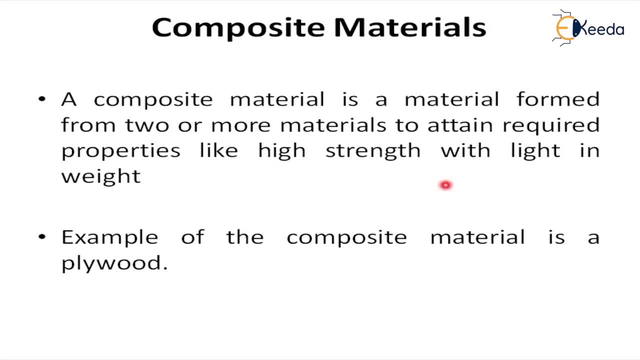 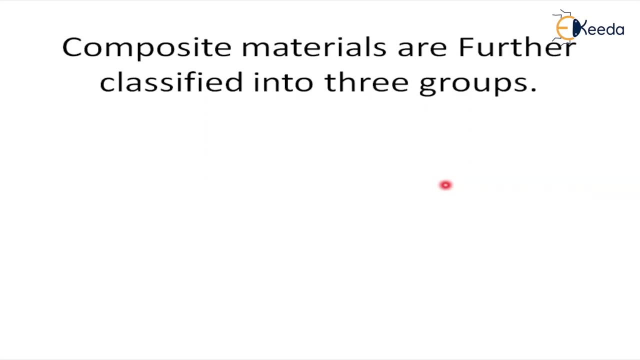 Most of the doors are made with plywood only. So that is the main application of the composite material. Suppose if you observe the regular or the so many applications, if you observe so many applications, there are number of applications for the composite materials, Not only in single area.